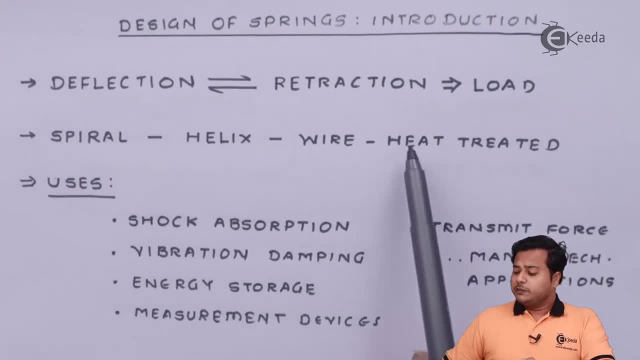 And that is why, in majority of the cases, the springs are heat treated or the materials that are used for springs are heat treated. Let us go for the usage. Different usage that we have for springs In industry are, first of is very important, that is, shock absorption. 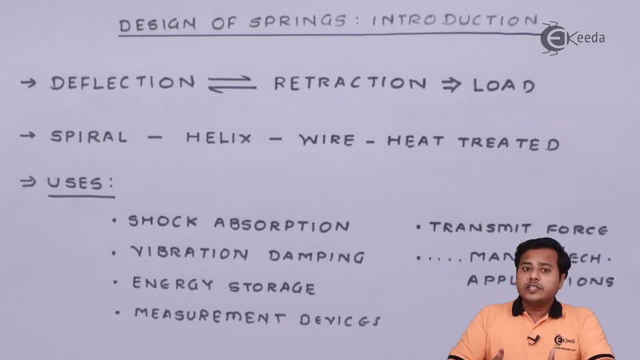 Whenever the shocks come into play or the loads which form the shocks, in order to absorb those shocks, we generally use springs. The next is vibration damping, If you see this properly major of the cases where the dynamic loads come into picture, where the vibrations are possible. 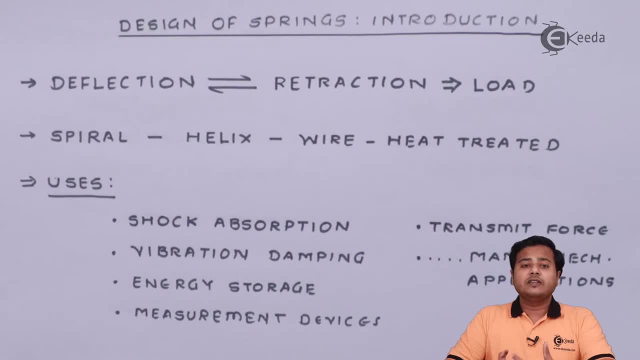 In that cases we need to absorb the vibrations, Otherwise they will be harmful for the machines and the operators. In majority of the cases, they use springs to damp certain vibrations or certain vibrations absorb certain vibrations. The next is energy storage. 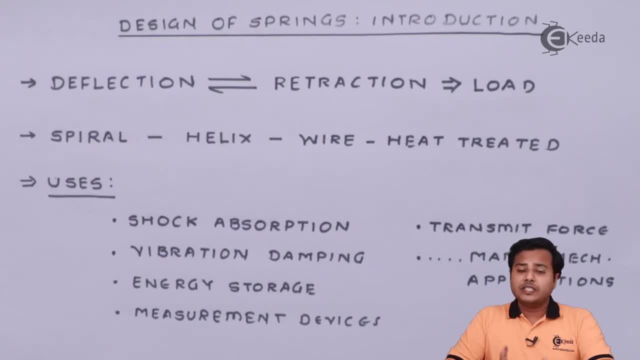 Now, this is a very day-to-day life example. You can use your wristwatch where we give, or the batteries where the batteries were not involved. In that case, we used to give certain rotation power to the springs In the form of energy. it used to be stored. 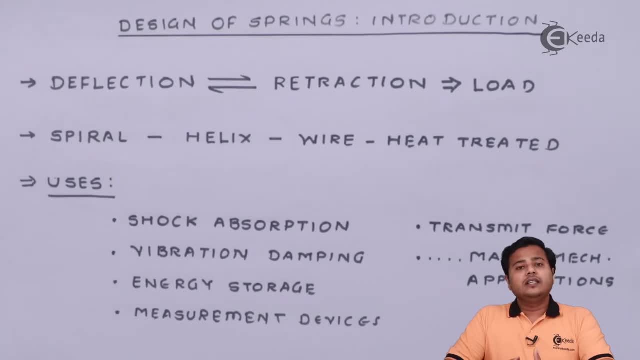 And the springs As they used to get unwind, the energy was utilized for running the wristwatch. So wristwatches or the coils are generally used, or the springs are generally used to store the energy also And release it at appropriate times. 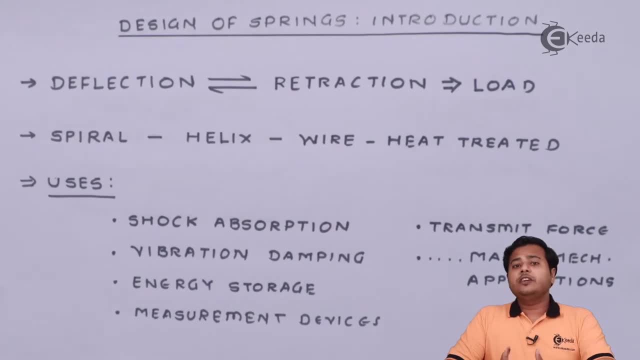 The next is measurement devices. Many of the measurement devices do use the same principle of energy storing and retrieving it back, And for that we need to use springs. The next is transmit force. Again, Many of the springs are used to transmit different forces. 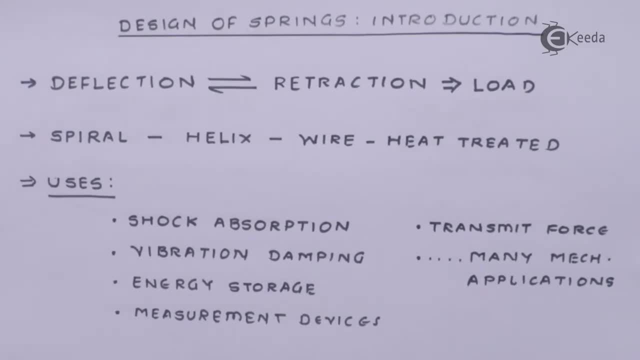 Again based on the storage of the energy or just simply transmitting the force, For example clutches. Clutches is a mechanical device. We already have studied this terminology in the subject of theory of machines. So in that case clutches do transmit different forces, or they resist the forces by means of springs. 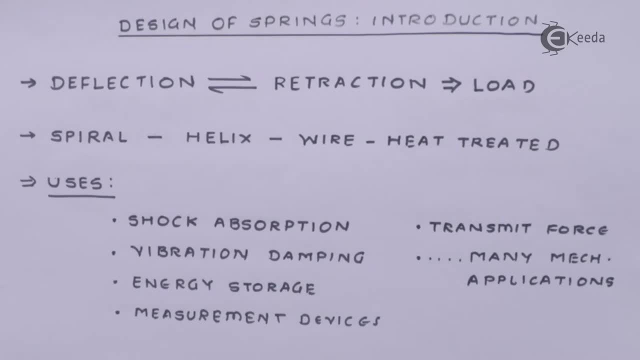 Last but not least, there are many mechanical applications where springs are used, Maybe a simple dynamometer or maybe something else that they generally use the transfer of the power, transmit the forces where springs are majorly used. So spring is a very essential, though it is small in nature, but it's a very essential part in order to work the mechanical systems. 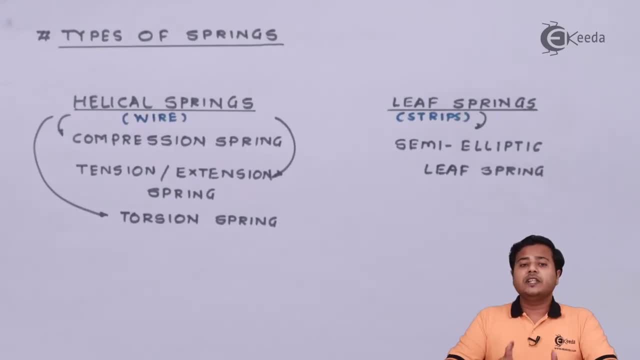 Let's move ahead. Let's begin with the types of springs. Now, since we are learning about the design and design aspects, we should know which are the types of springs. Now. there are various types of springs, of course, specialized one as far as the industries are concerned. 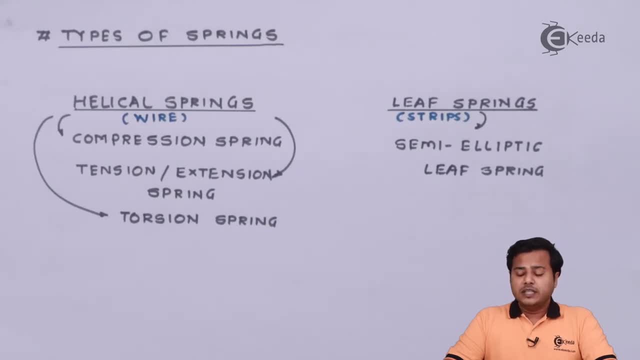 But, as per your syllabus, we are going to look at only two types. The first type you can see is the helical springs And the second type you can see is the lip springs. Now, helical springs are generally made up of wires and wires to have the cross section circular in majority of the cases. 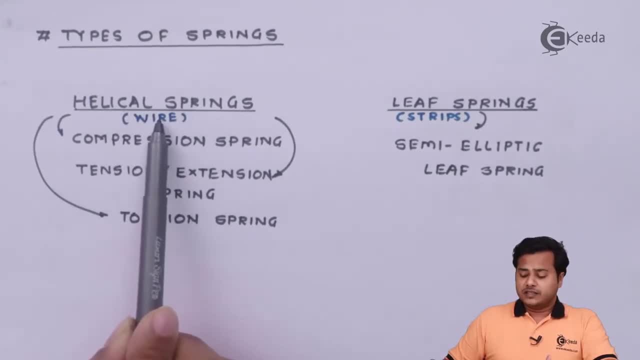 And that's why helical springs are made up of wires. The next thing is there are subtypes of helical springs. Helical springs are generally used as the compression springs, or they are used for the tension or extension springs, or they are used for the torsion spring. 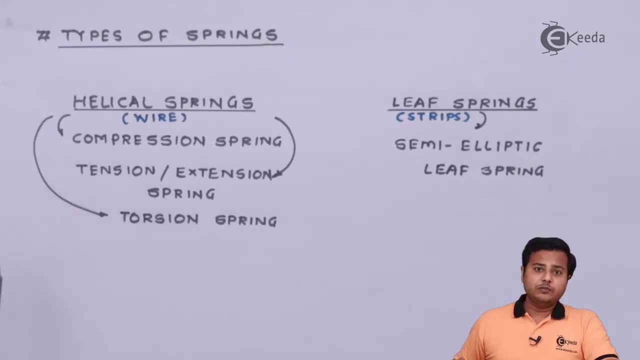 So these are basically their application point of view. The next is lip springs. Now, lip springs are made up of different materials, or the strips of materials, or metals, you can say. And the general application point of view, The general form of lip spring is semi-elliptic lip spring, where the curvature goes into the elliptical way. 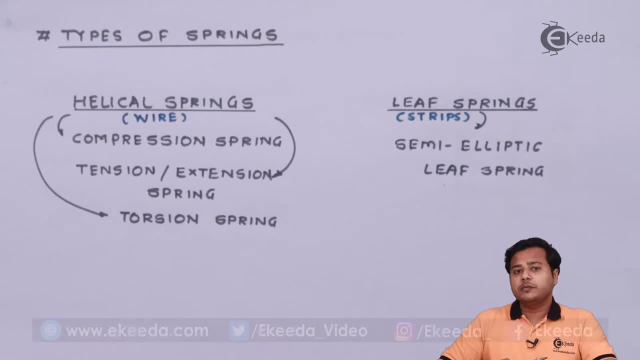 And they are semi because the only half portion of them is utilized for storing or whatever the purpose they are being used. Of course we are going to do their detailing afterwards, We are going to look at the design aspects afterwards And then we are going to look at the numerical. that can be solved. 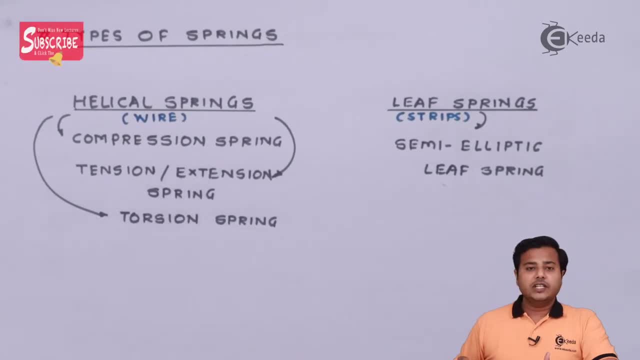 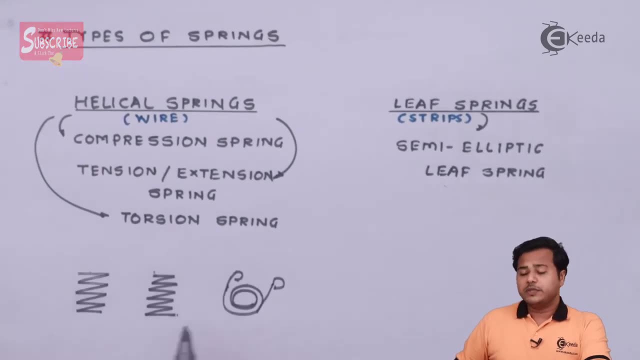 So these are the important things. So when these types are distinguished, let us look at the application point of view. Let me quickly draw them. So this is a kind of spring. Of course they are simple springs which are shown when the load which is acting has the compressive nature. 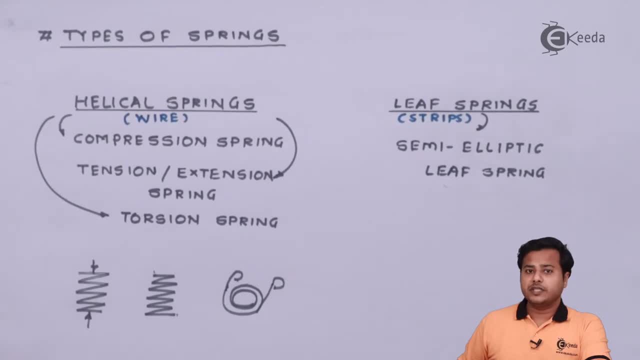 The springs used are basically called compressive springs When the nature of force is such that the force will act away from the spring or they act towards the end points. In that case the spring utilizes, called tension spring. The spring utilizes called tension springs or extension springs. 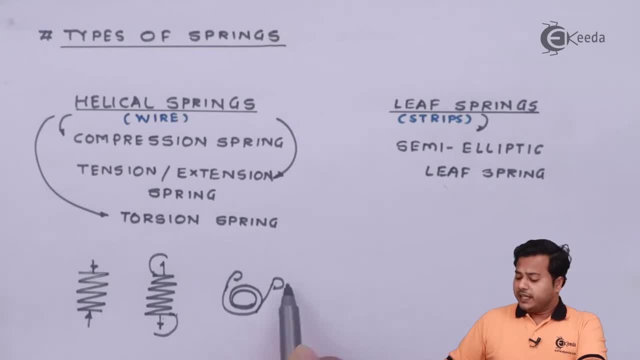 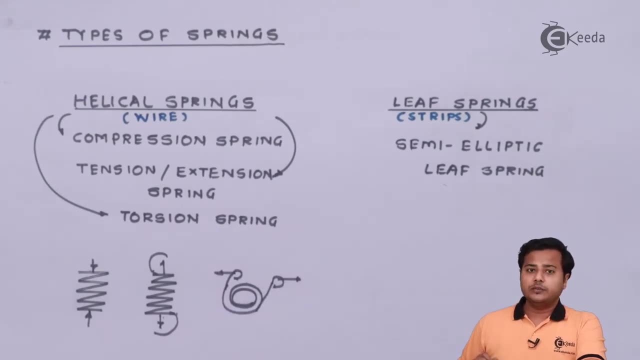 The last but not the least, it is the same spring, But in that case the forces do act in such a manner that they induce the torsion inside the given body of the spring, And that is why they are called torsion springs. 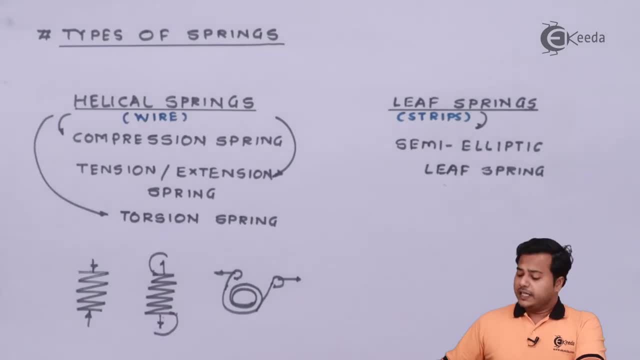 This is the main type. Whereas the lip springs, they have different lips. like them, The lips are nothing but the metahecal strips which have undergone certain changes. So certain many lips, or the strips, they are brought together so as to sustain different loads. 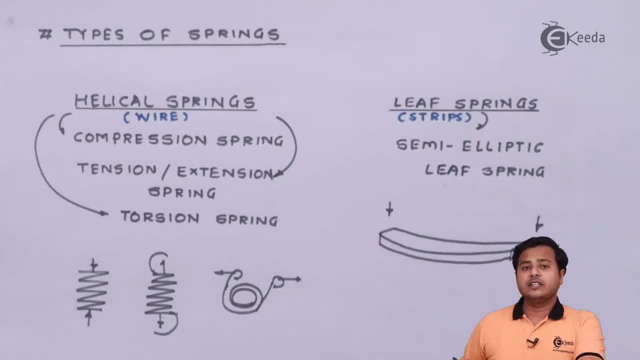 All these lip springs are going to sustain transverse loads. in that case, Like in this case, we have compressive tensile and torsion. In this case, the loads that are going to act on are torsion. Mainly, lip springs are utilized for the heavy automobile vehicles for their suspension systems. 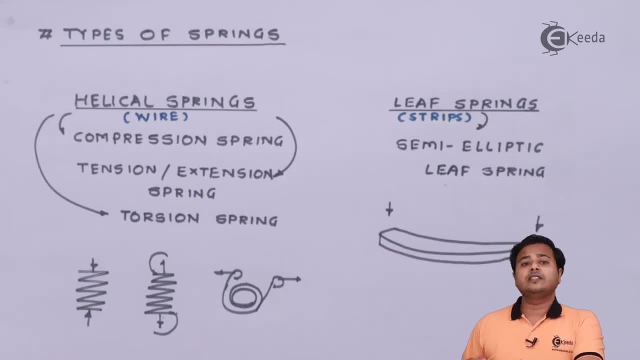 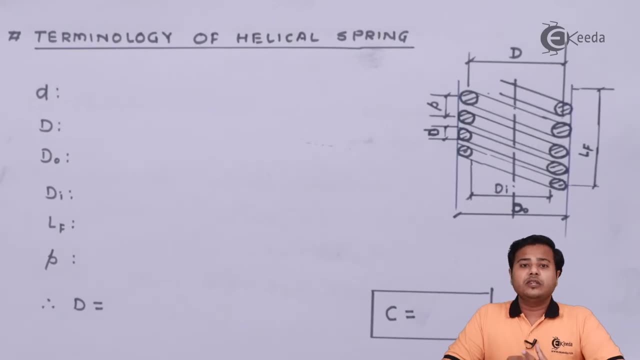 Because in that case it is very difficult or it is not doubtful It is very difficult or it is not that feasible to use the helical springs. Let's move ahead. Now there comes an important thing, which is called terminologies, Since we need to understand different design aspects of this particular member. 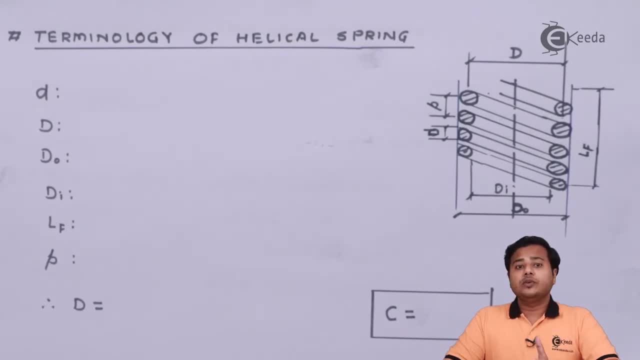 we need to understand various terminologies or various notations they use for this particular spring. So let us begin with the helical spring. As you can see on the screen, there is a schematic given for this spring. It is a cross-section given. 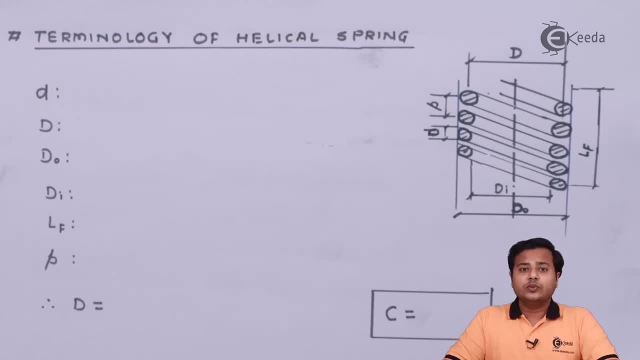 And you can see the spring wires. on only one side, Only one half, are shown. Let us look at them. If you see this particular structure, they are nothing but the cross-sections of the springs. Of course, they are circular in nature on both sides. 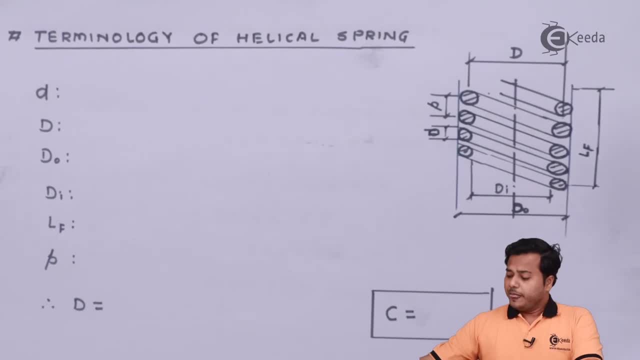 This is the axis about which they are going to be symmetric. Let us start with the length. The total length from the beginning of the spring till the end of the spring, no matter where the end is, is called the free length of the spring. 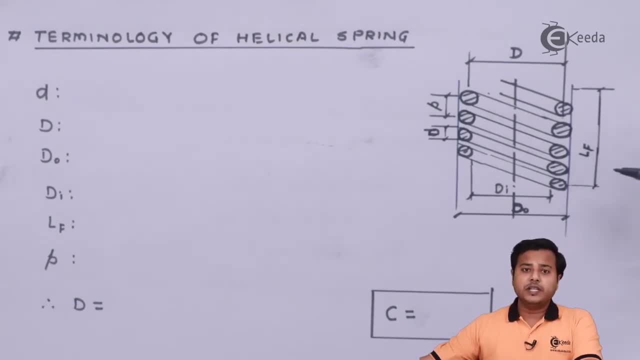 So free length is the maximum length of the spring which is possible when there is no force acting on that particular spring. The next thing is the small d. Small d stands for the diameter or the cross-section diameter of the wire which is used for that particular spring. 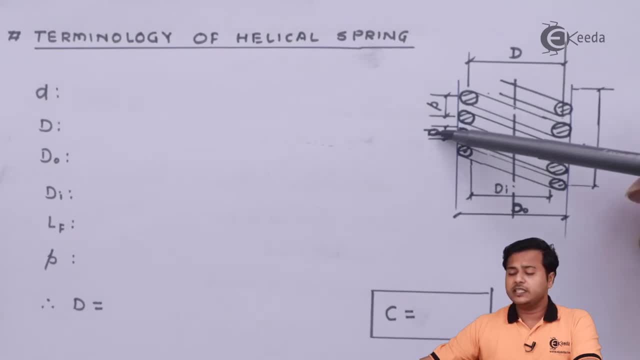 So in that case you can see this circular cross-section. It is nothing but this small d. Next thing comes is the diameter d, capital D. It is nothing but the mean diameter of the coil. Now, if you see from this end to this end, 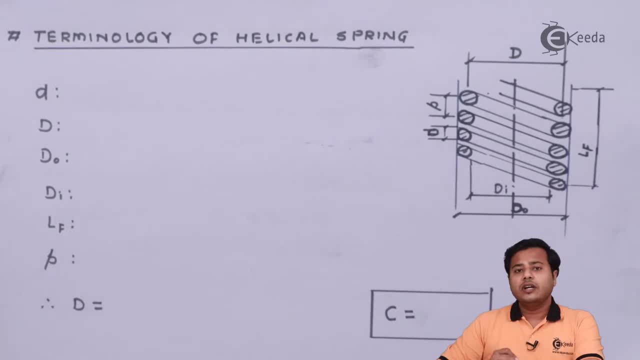 this particular round or this particular turn, is called coil. So this coil, the mean diameter, is called capital D. Now there are two different terms associated: inner diameter and outer diameter. Now, inner diameter, if you see, will be the distance between the innermost layer of these cross-sections. 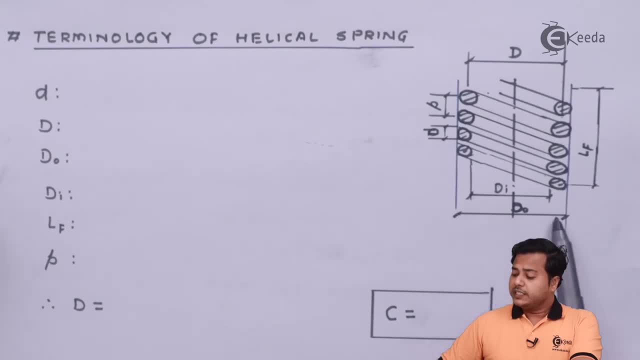 Of course, circular- they are in nature- And outer will be the distance between the outermost layer of this particular dimension. The next and last terminology which is very important here, is pitch. Now, pitch, if you see, is proper the distance between two consecutive points of the spring. 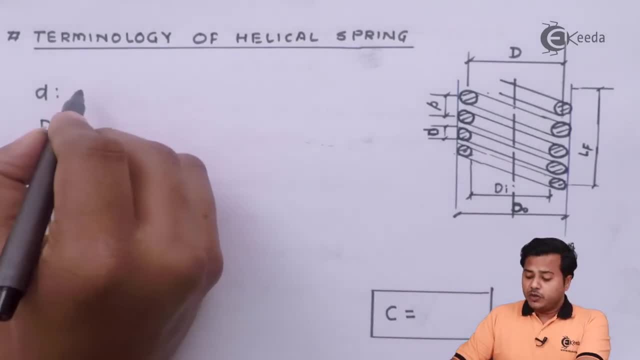 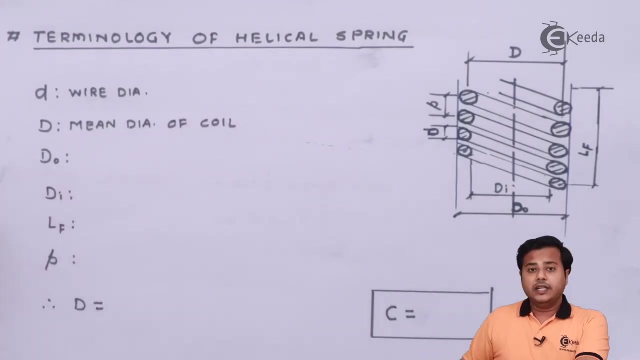 So let me quickly summarize this: Small d is nothing but the wire diameter. Capital D is the mean diameter. Of course it is associated with coil Do. that is the outer diameter. That is the outer diameter Again, of coil. 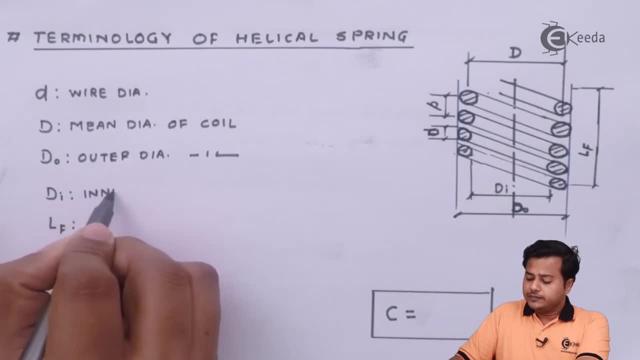 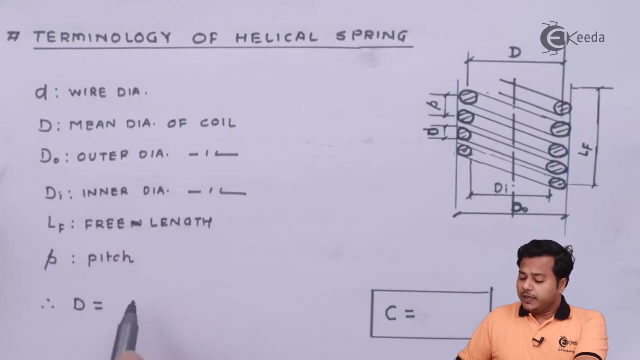 And di is nothing but inner diameter. Again, associated with the coil, There comes lf, that is, the free length of the spring. This is the pitch, And So that the D will be given by the bisection point of the outer diameter and the inner diameter. 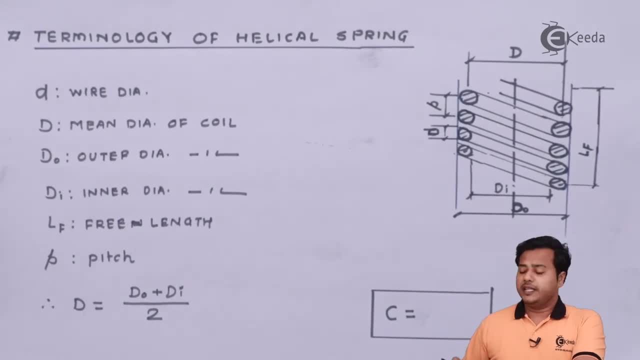 There comes another particular term that is called spring index, which is given by C. Now, spring index is nothing but the ratio of the mean diameter of the given coil to the wire diameter of the given coil. We can see the mean diameter, which is: this is always greater than smaller diameter. 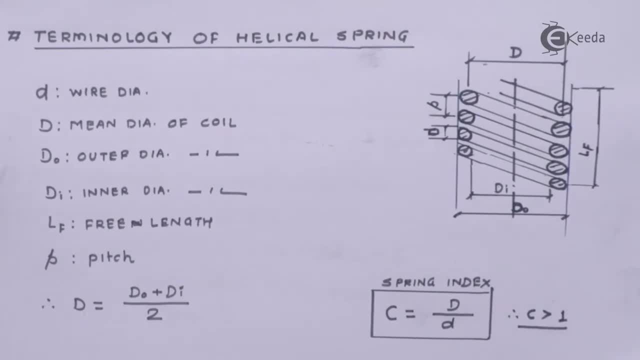 And hence C will be always greater than 1.. Now this factor spring index is going to be used frequently whenever we are going to solve the numerical based on the design of this particular spring. So these are the some of the important terminologies which are going to be used in the helical spring. 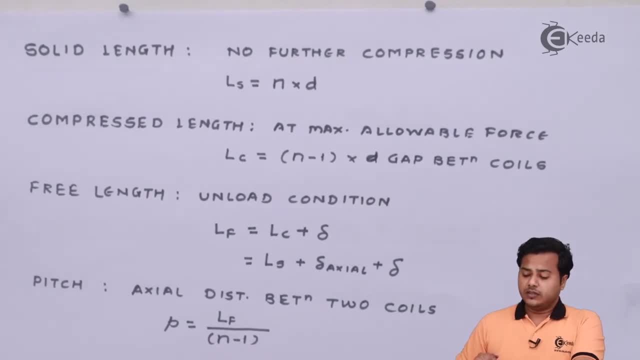 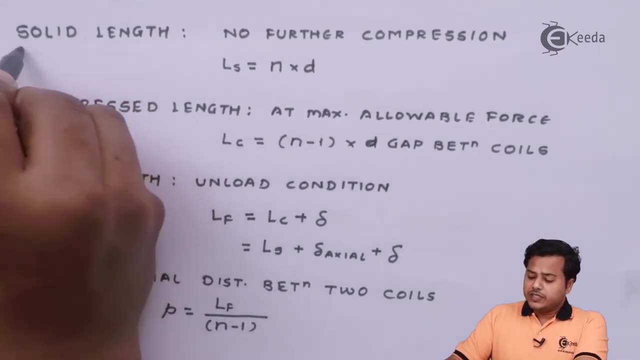 Let's move ahead with some another terms. I will not call them terminologies, but terms which we are going to use for that particular inspection. So the first one is the solid length. Now, solid length is no further compression is possible. 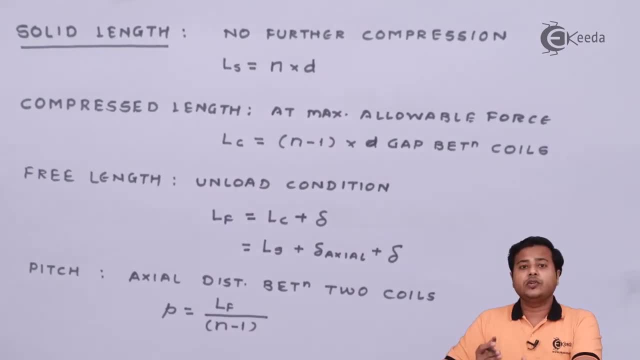 Now, students, when a spring is compressed, in that case the coils will touch each other, Since that is metal and that is not a plastic material. it will not deform beyond this. So when the maximum force, maximum possible force. 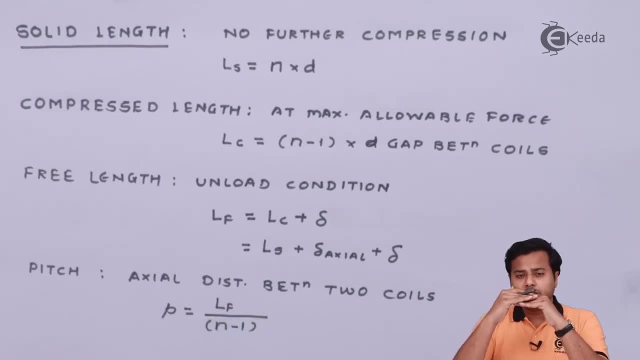 is applied on the structure, then the coils will touch each other so that the length form will be a solid where no further compression is possible. So in such case the length obtained is called solid length And it will be given by n into d, where small n is the number of coils, into d is the diameter of one wire. 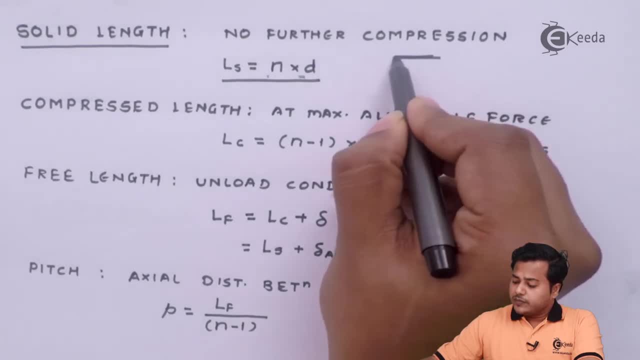 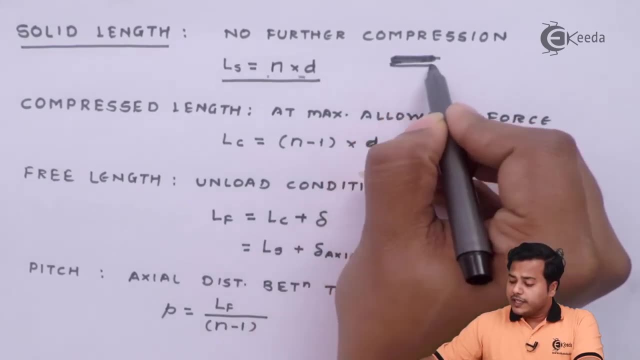 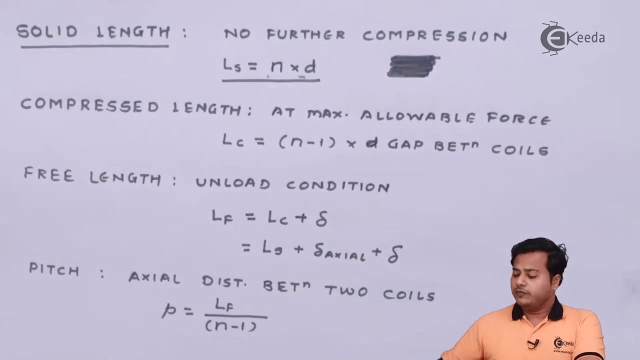 So if you need to draw the compressed structure, let me call. this is the first coil. The second coil is attached to it. Since they are closely attached, there is no gap between them. Let me add the third one, fourth one and so on for the n number of coils. 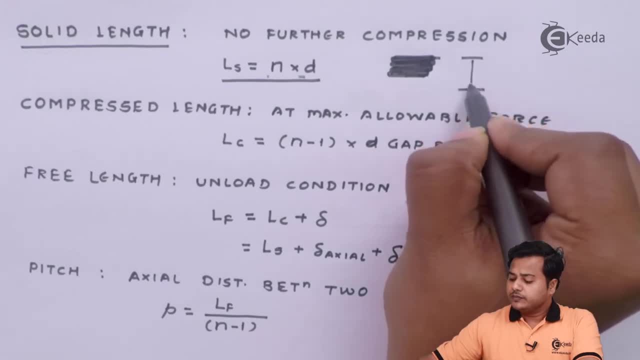 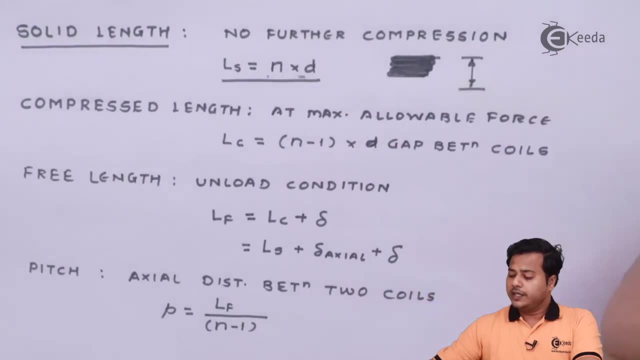 And that's why this solid length up to n number of coils will be n, which is 1,, 2,, 3, 4 and so on, up to n, into one diameter of any respective coil. Next thing is compressed length. 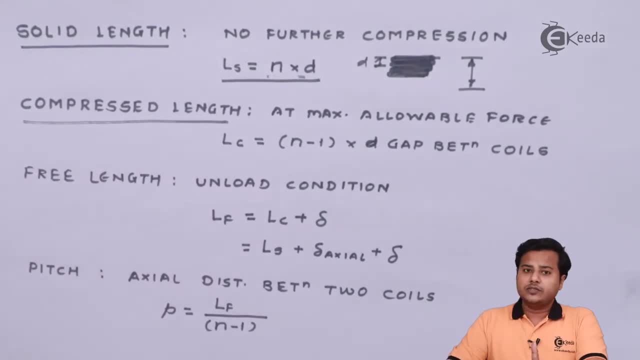 Now there is a minute difference between this compressed length and solid length. Both are obtained when they are compressed, no doubt in that. But compressed length is obtained when a maximum allowable force is applied. It's not the maximum possible force, It's the maximum allowable force. And you should understand that maximum allowable force has to be smaller than the maximum possible force. So when maximum allowable force is acted upon by the spring, naturally it will compress, but it will not compress to the full extent. There will be some gap maintained by two coils. 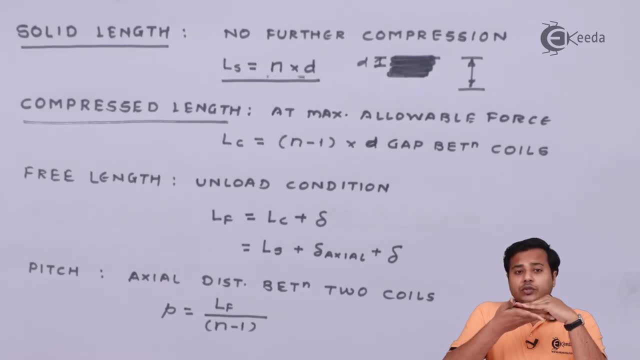 And considering this gap, whatever total length comes out to be, is called compression length. So if you need to draw this schematic, it will be somewhat like this. Let me call this as the first coil. There will be certain gap between the second, third and so on. 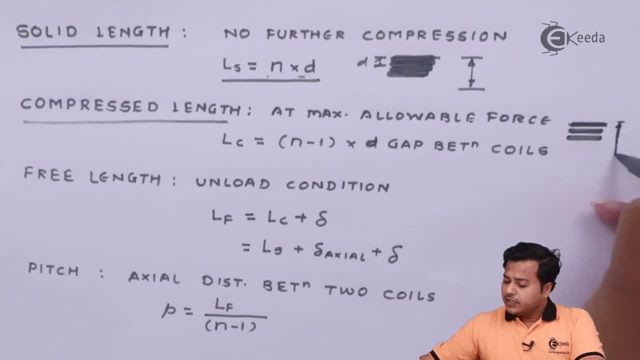 so that from the first end up to the last it will be the compressed length And if you see logically it will be given by n minus 1, total number of coils minus 1, because we are considering this time gap also Into gap between the coils. 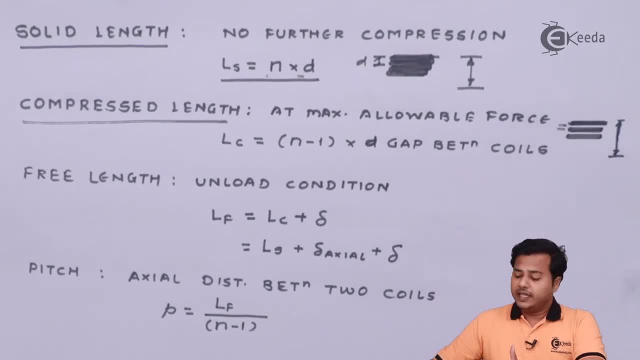 Now see if the gap is 1 to 2 millimeter. In that case we have to consider this gap into the coil minus 1 or the number of coils minus 1.. That will give me the compressed length. The next term is free length. 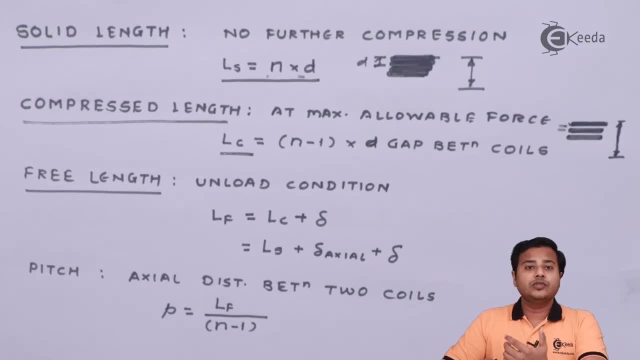 Now, free length is the length of that particular spring where there is no load acting. Since there is no load acting, it will undergo its natural length, which is possible for the spring to obtain, And that's why it is called unload condition. 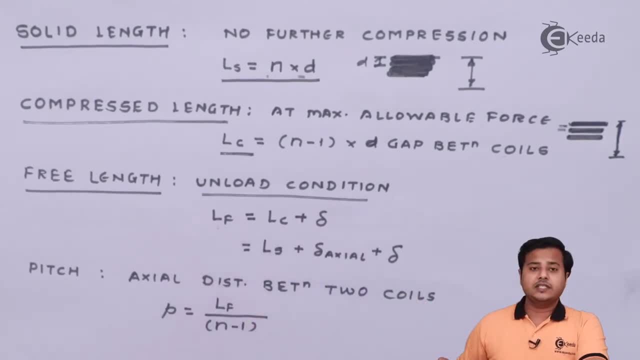 So in that case, the free length, which is designated by LF, will be given by the compressed length plus the maximum deformation possible for a spring, which will be also given by the solid length plus the maximum axial gap. That is nothing but this, two plus the maximum deflection possible. 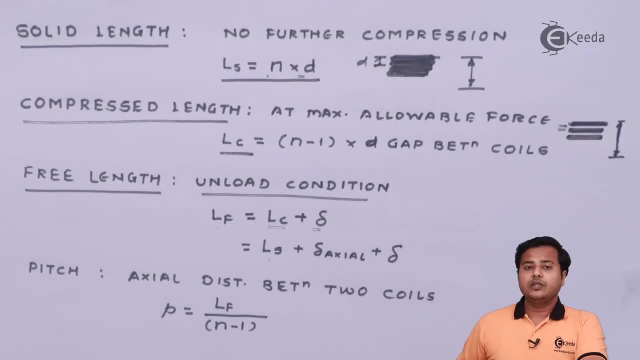 So either of this empirical formula we can use to find out the free length. Let's go to the next, which is very important, like we have discussed, Pitch. Pitch is the axial distance between two consecutive points on a coil. So it is the axial distance between two coils or the consecutive points on the coil. 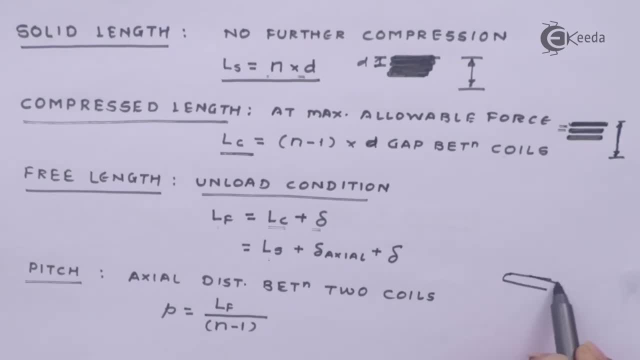 For example, if this is how the spring is structured, I have shown only the cross section. The other side of spring is not shown. So in that case, this is the first coil and this is the next coil. So in that case, these two points are same. 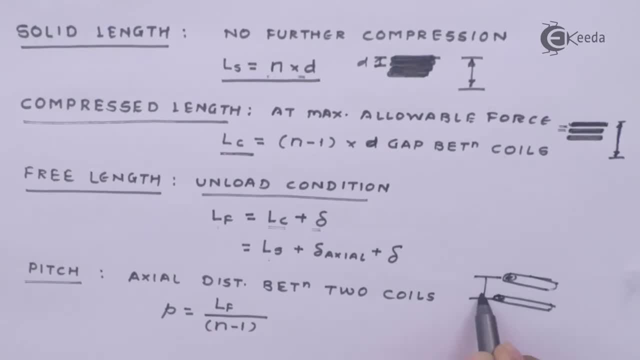 I'll call them consecutive points, So that the distance measured along the axis or parallel to the axis will be called pitch, And hence pitch will be given by the free length of a coil divided by this particular term, which is number of coils minus one. 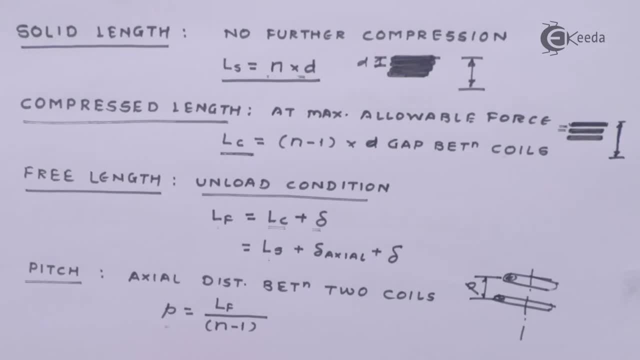 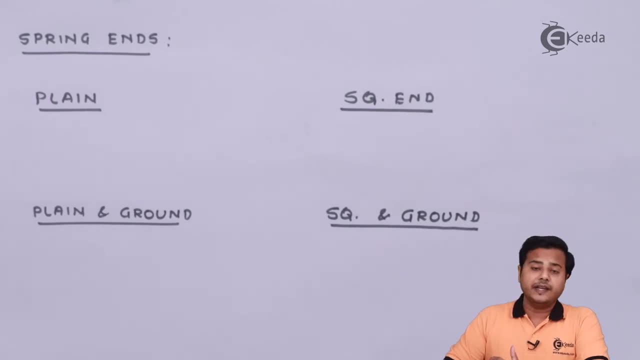 Because we are not considering the last coil in that case, because we are taking the difference between two consecutive coils. So next important thing that we need to understand is: the spring ends Now. spring is a continuous member which has certain constraints for its dimension. 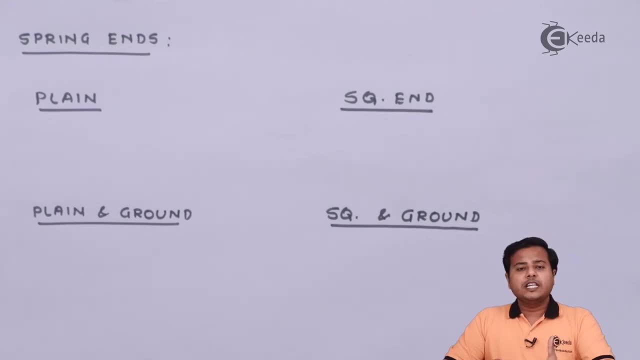 So somewhere it has to end, But it's not a skipped end or it's not a random end. We have to pre-define the end so as to place this spring properly in the given mechanical system, Because spring has to interact with multiple sections, multiple fragments, multiple surfaces. 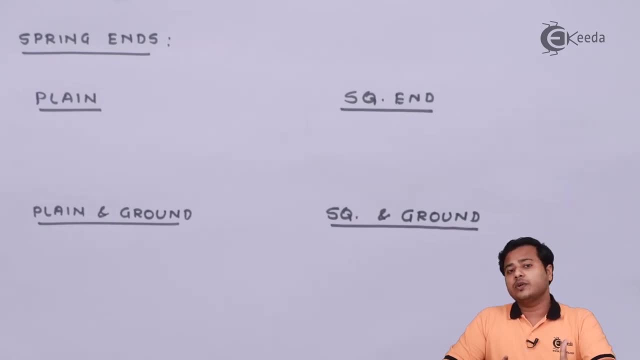 And in that case we should have a provision so as to fix this spring properly, And that's why certain ends are used, Four such popular ends we are going to look at. The very first end that we see is the plane end. Let me draw this schematic of a spring. 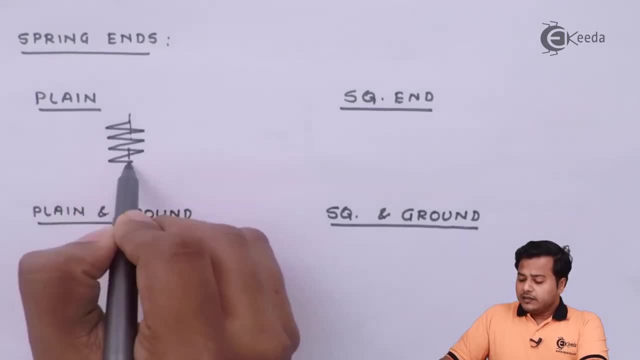 If you see, the aims are fixed with certain angle again, So it continues with the same angle. Of course, that angle is called helix angle. The particular angle that it makes with horizontal is called helix angle, Beta- generally they call it. 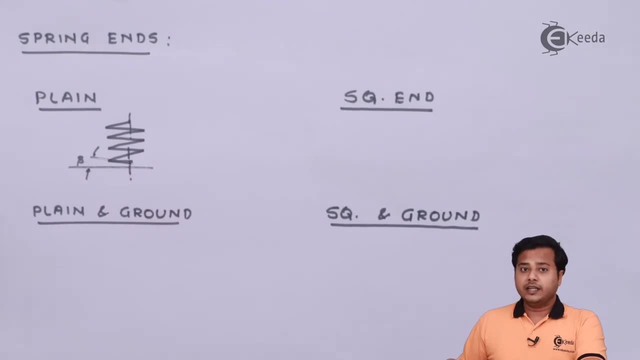 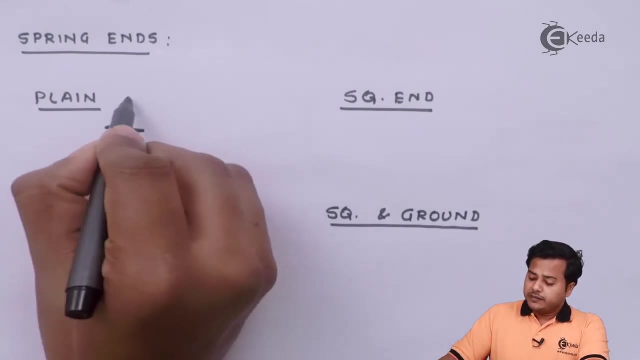 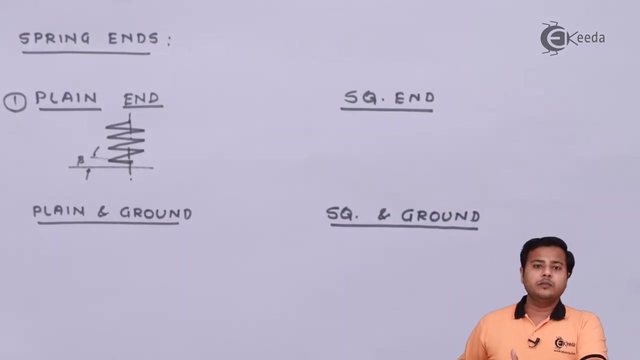 So the spring which has the end where the helix angle is maintained, such a spring will be called a plane spring Or it will call a plane end spring. So it's the most simple form of the spring end. The second form is little modified and which is called plane and ground. 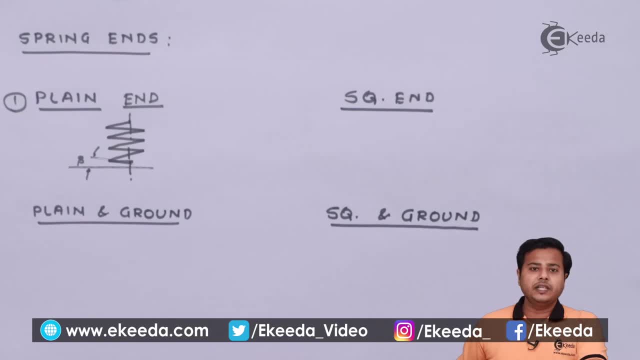 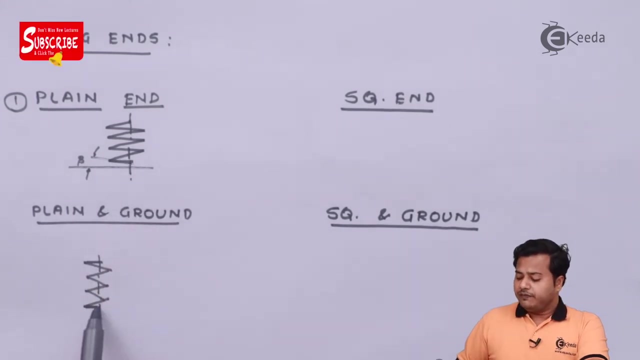 Ground term is used for the flattening of the given end. So in that case the end will look like, If you see, unlike the first type, the ends are flattened. They don't have the helix angle maintained there, So that this is a horizontal one in this case. 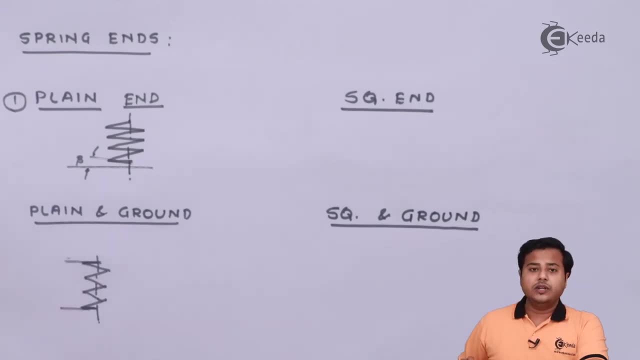 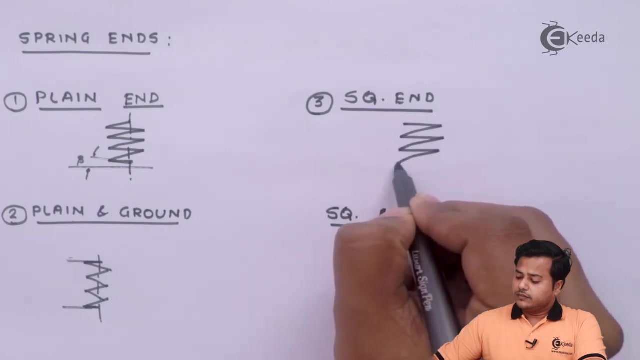 And that's why they are called plane and ground end of the spring. So this was the second type. The third type is quite different, where it is called a square end. In such case, if you see it's not midway, It is taken to the end points, where the ends are properly done with the square kind of thing. 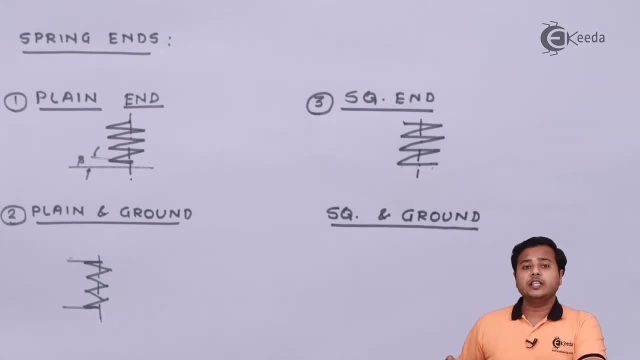 The next modified version of square end is nothing but square and ground. Where, again, the square ends are made ground, If you see properly. they are particularly ground where they are cut in the shape where it is required, And that's why these are the four different spring ends that may have to be used. 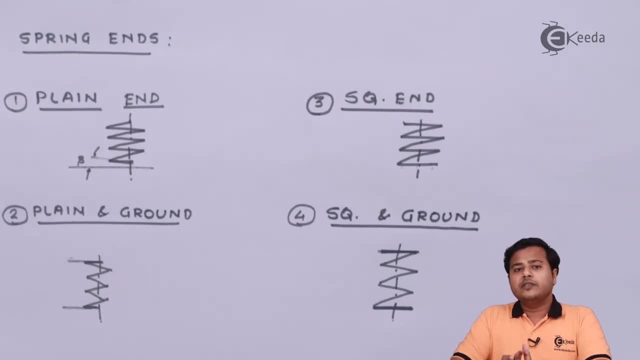 So it's a small portion of the numerical that we are going to look at, Where at the end we have to predefined or we have to select a predefined given kind of end Which has a small impact on the further part of the numerical. 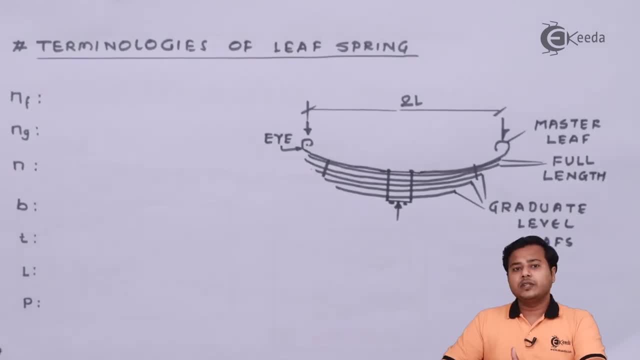 Let's move ahead. We have arrived at the last segment of this particular lecture, Where we are going to look at the terminologies that are used for the lip spring. We have seen so far the terminologies that are used for the helical spring. 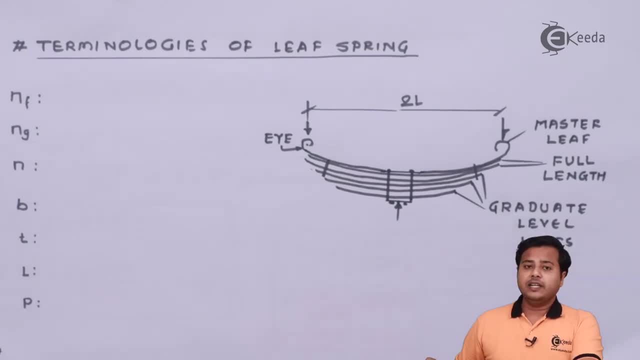 But this is for the lip spring. Now, this is how the schematic of the lip spring is given. I have drawn just a schematic. It's not a proper diagram, But I think it is explanatory. You can see, the different curves are nothing but the lips. 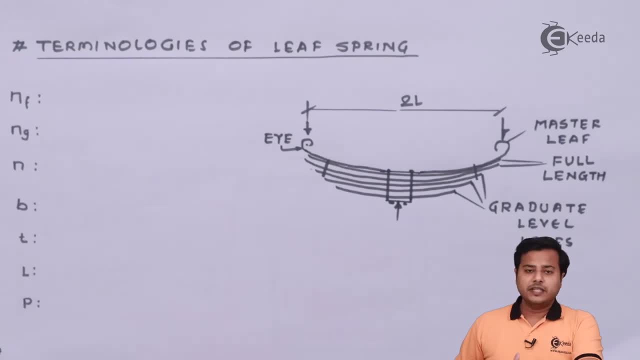 They are called lips because they appear to be lips. They are made of metals And we already have seen the cross section. I will draw it for you again. These are basically metallic strips which undergo certain bending. Now the layers in which they act. they have got certain significance. 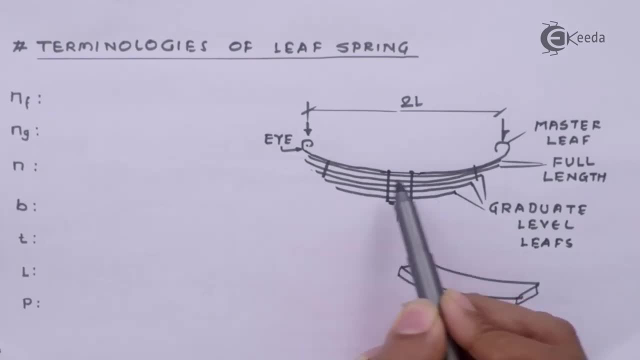 If you see properly. of course they are symmetric about both the layers. The topmost thing is bolted properly And the fours do act on this. Of course these bolts do represent a fixture where the spring is going to be fixed. 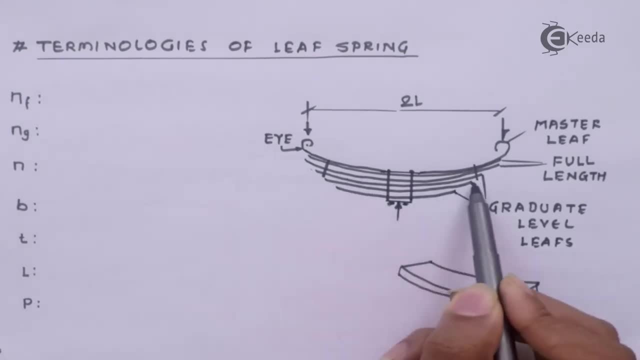 The layer one, the next and the next layer. if you observe it properly, the lengths are going on increasing one by one, And that's why they are called graduate level lips. Now that depends upon the application: how many graduate level lips we have to use. 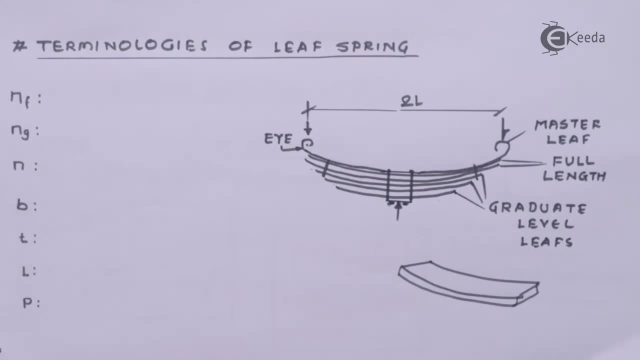 Sometimes they can be two, three, four or five. also, As soon as the graduate level lips are end, they will start to equal length lips And these are called full length lips. So these are the fullest length which is possible And they are equal in length. 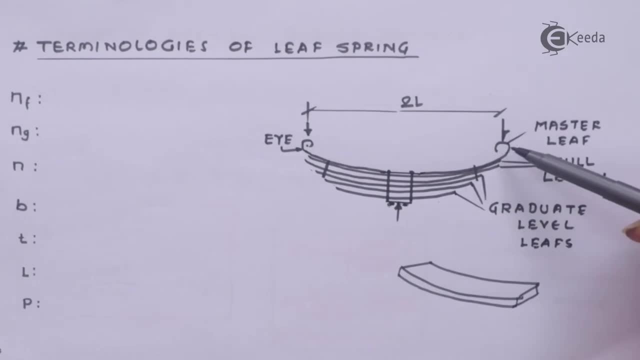 There comes the last lip, which has got different bend ends, And this lip is called master lip. The master lip is going to be attached to the application to which this spring is going to be attached. Now, the forces that do act on this spring are called P. 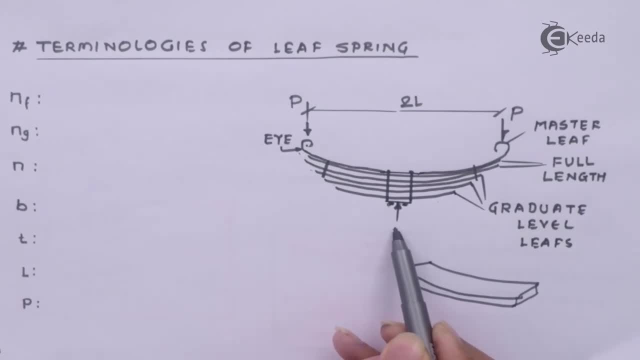 Let us call them P on either sides, So that the reactive force or the supportive force will become twice the P. The last terminology that they use is this: bend end of the master lip is called I. It's called an I. So these are the important terminologies that we are going to look at. The last thing is between two I's. their center to center distance is defined as twice the length. Now let us look at them quite rapidly. The first one is the NF. That is nothing but the number of full length springs, Number of full length lips. 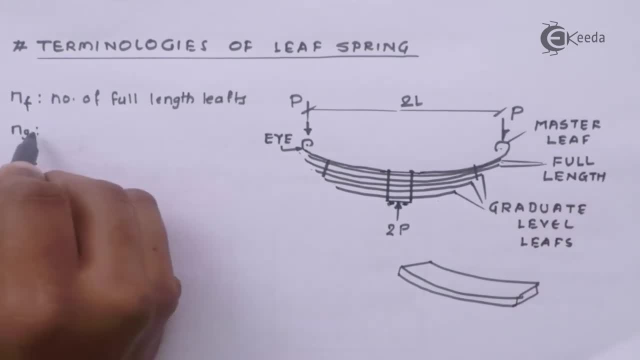 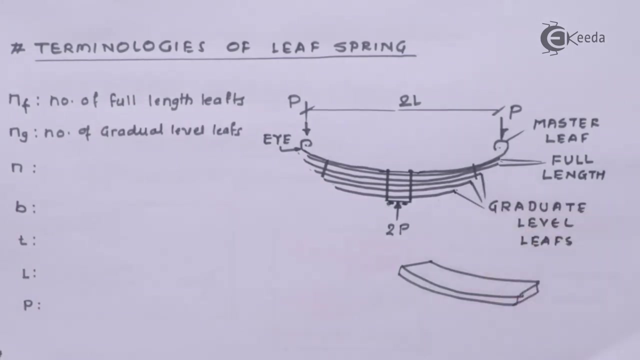 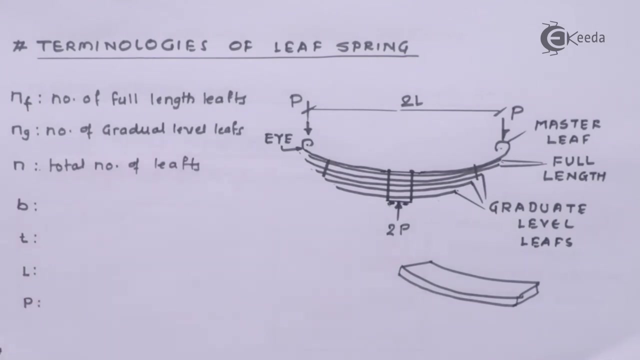 In our case there are only two, one and two. The next one is NG, where it's called as number of number of gradual level lips. In our case they are one, two and three. The next one is the total number of lips. 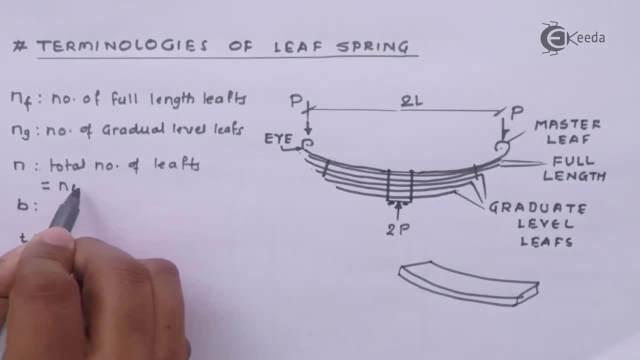 So in this case it will be equal to NF plus NG. The next is the D, which is nothing but the width. So in this case, this particular dimension is nothing but the width of a spring or lip. The next is the thickness.